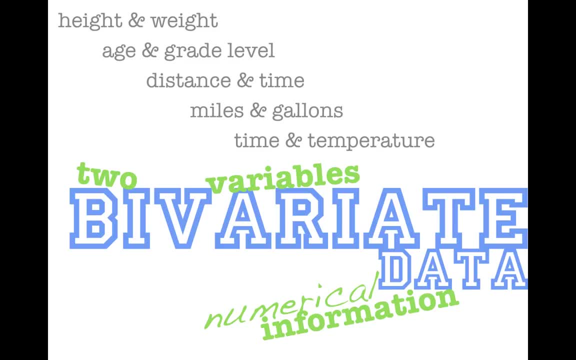 or miles and gallons, or time and temperature or any two variables. But whenever you have two variables and you have data about each of them, you're going to have a lot of information. We have what we call bivariate data. Now I want to talk about the Orange County Fair. 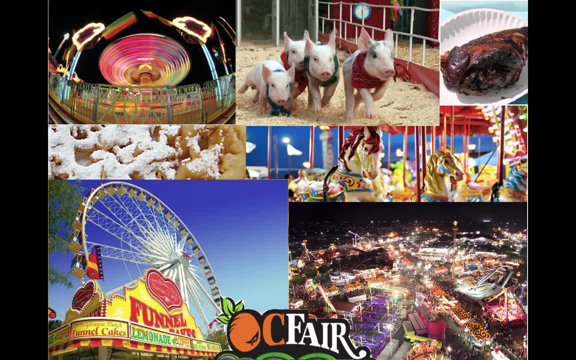 You ever been to the Orange County Fair? I bet you have. When you go to the Orange County Fair it's a little different than going to some other amusement parks, because first you have to pay some money to get in the gate of the fair, just to go there. Then once you're inside, you probably 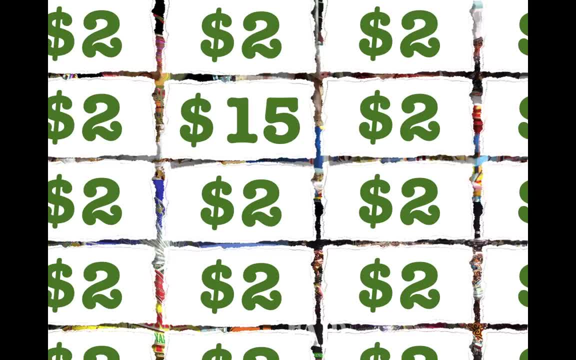 want to go for some rides and each ride costs more money per ticket. So let's say you pay $15 to get in the gate of the fair. You have to pay $15 to get in the gate of the fair. You have to. 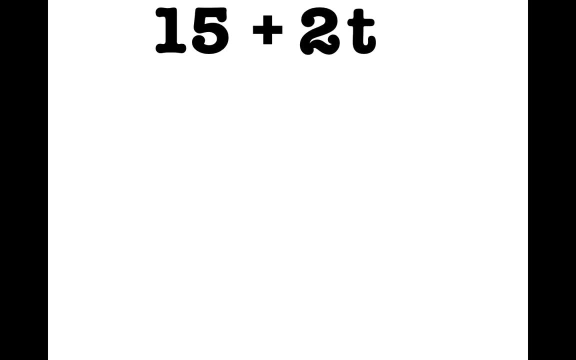 get in the gates. Plus you pay $2 per ticket. This isn't bivariate yet, because the only variable is the number of tickets that we bought, But it really is bivariate because the other variable is the cost of going to the fair, And the cost of going to the fair is dependent on another variable. 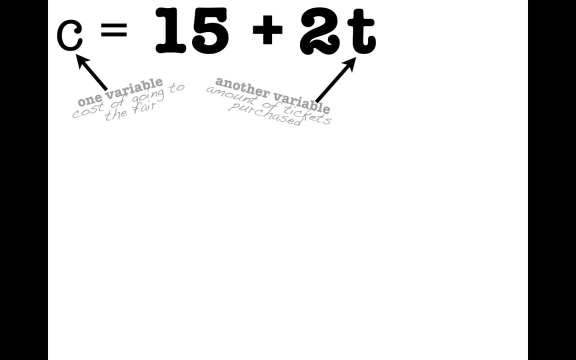 the amount of tickets purchased. So this is an example of bivariate data. Now, bivariate data loves to be displayed in a table, like an input-output table, where we could put the dependent variable over here and the independent variable over here, Or we can. 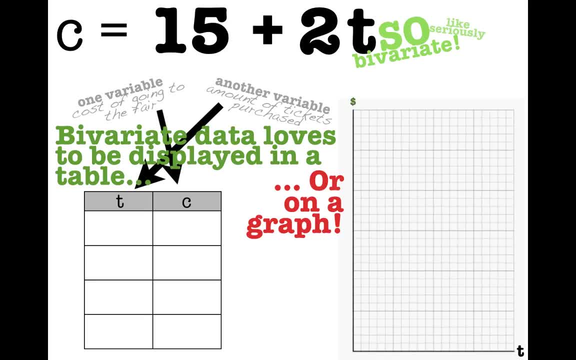 take that bivariate data and display it on a graph. Bivariate data loves to be displayed on a graph as well. So let's say you put the number of tickets on the x-axis and the number of dollars on the y-axis and we start plotting some points. For instance, if you buy no tickets, it's just $15. 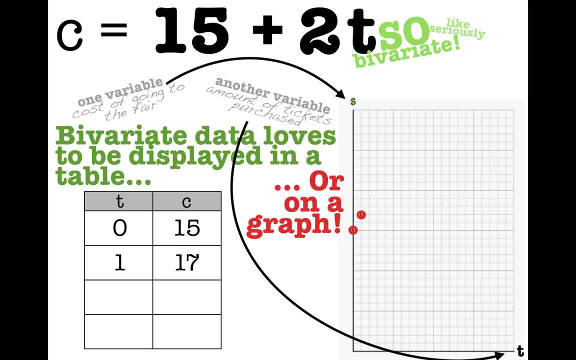 to get in the door and you've got a dot there. If you buy one ticket, that's $2 more, so that's $17.. If you buy two tickets, that's $4 on tickets plus the $15 to get in the door, for a total of $19.. 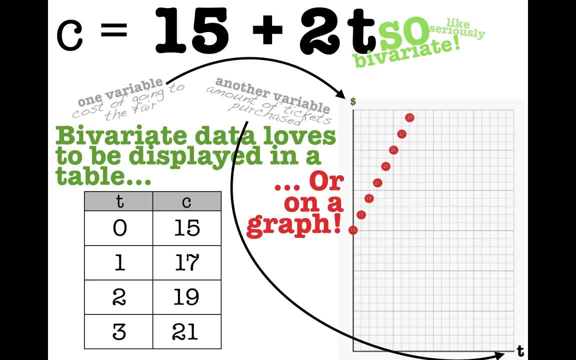 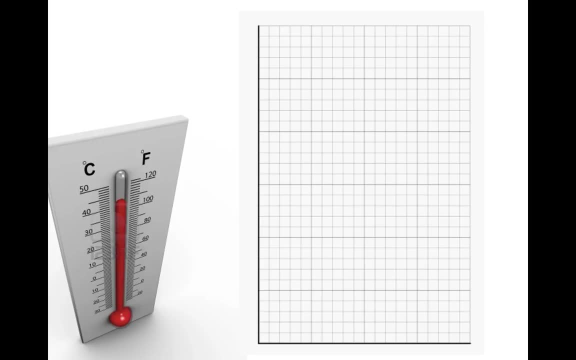 And what we've got here is basically a bunch of bivariate data. that could keep on going and going and going. This bivariate data happens to be perfectly linear, but not all bivariate data. For instance, let's say you collected some bivariate data where your two variables were. 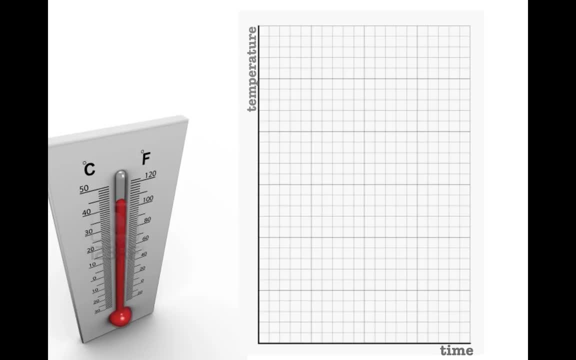 temperature over time. Like, let's say, you woke up in the morning and it was 40 degrees, Then a little later it warmed up to 44, and then to 50, and then to 54,, but then it kind of stayed 54. 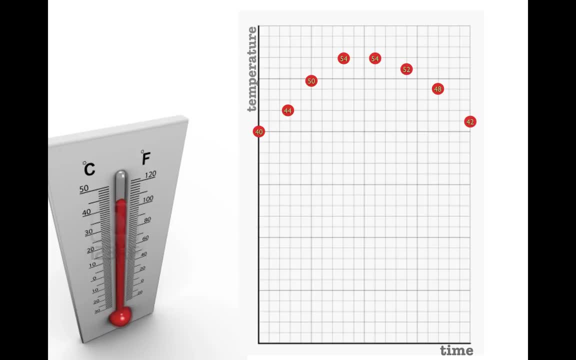 until it eventually started to cool off later that evening. This would still be bivariate data, even if it doesn't make sense. So let's say you collected a bunch of bivariate data and it's just $15 to get in the door, for a total of $19.. So let's say you collected a bunch of bivariate data and it's just $15 to get in the door, for a total of $19.. I' t going to make a straight line because it's still data that has to do with two. 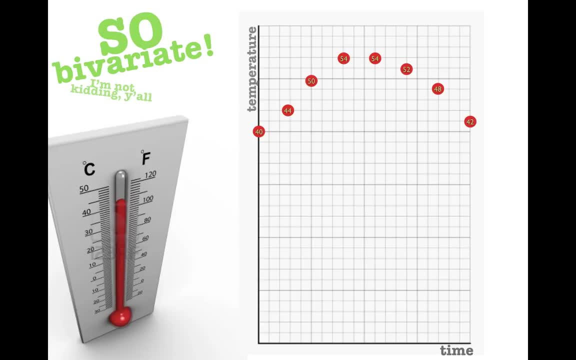 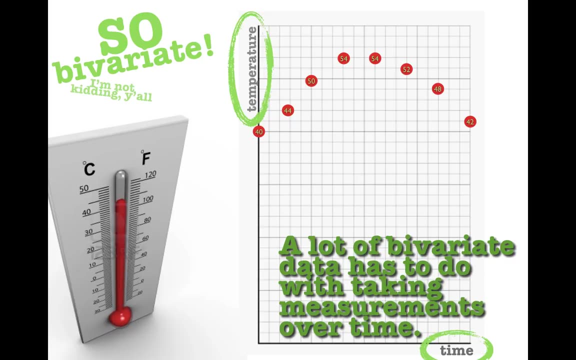 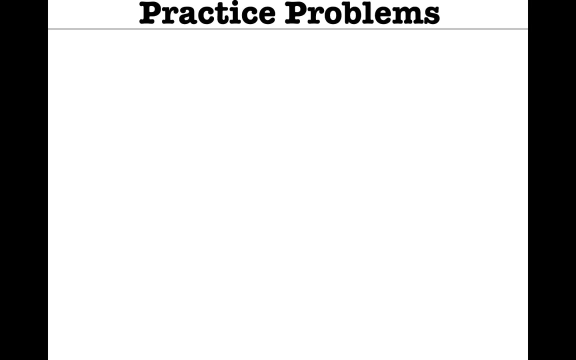 variables, time and temperature. A lot of bivariate data, by the way, has to do with taking measurements over time. So often you will see the x-axis labeled with some kind of time measurement. All right, you've heard a little bit. 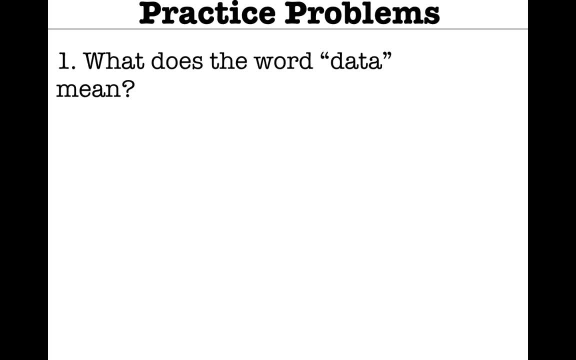 about bivariate data. Answer these questions please. What does the word data mean, What does the word bivariate mean, And name two ways that you can display bivariate data. Okay, now that you've unpaused the video, we're going to move on to talking about scatter plots. 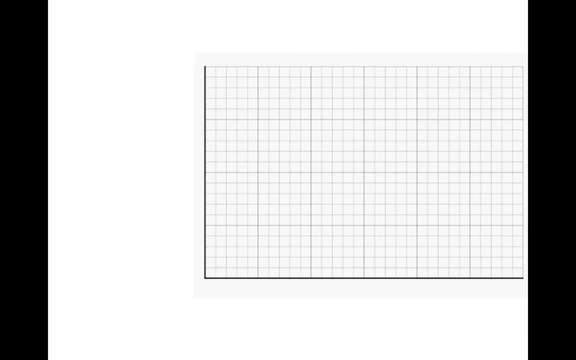 What is a scatter plot? A scatter plot is when you plot some bivariate data. So let's talk about height and weight- No fat jokes, because the height and weight that we're talking about here is going to be little kids going to the doctor's office. 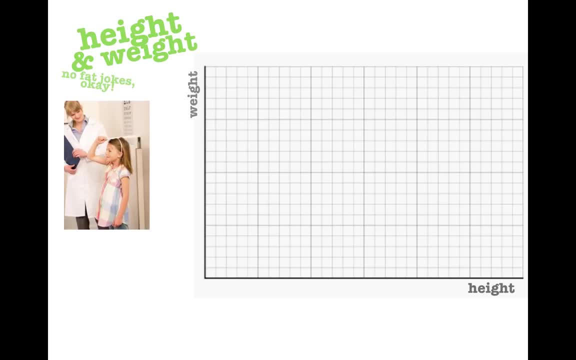 and getting their height and weight measured, and it's not cool to make fun of little kids. So let's say we put the height on the x-axis and the weight on the y-axis and we start measuring some kids. So the first kid is 30 inches tall and 40 pounds. 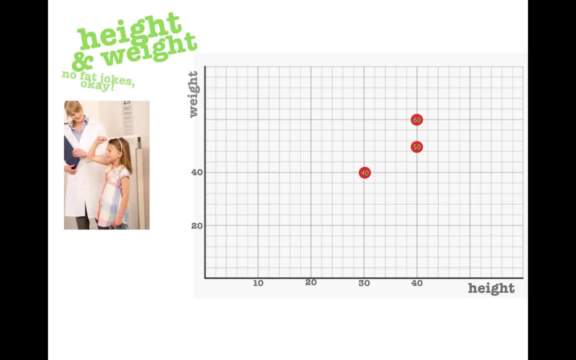 The second kid is 40 inches tall and 50 pounds. The third kid is 40 inches tall as well, but heavier- 60 pounds- And we get scatter plots. So we're going to make some more kids of various heights and weights throughout the rest of the day. 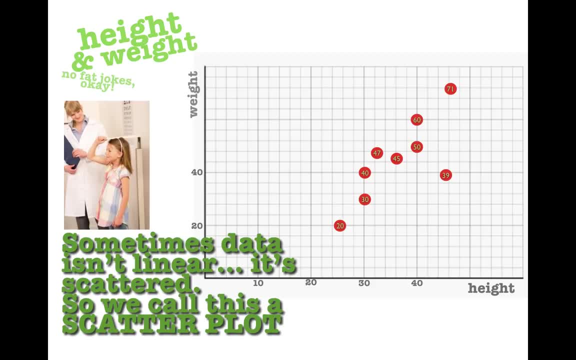 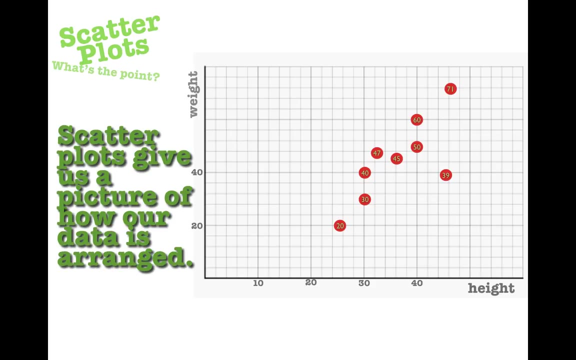 Sometimes data isn't linear. It's scattered all over the place. So we call it a scatter plot because the dots are kind of scattered all over the graph. What's the point of making a scatter plot? The point of making a scatter plot is that it gives you a picture. 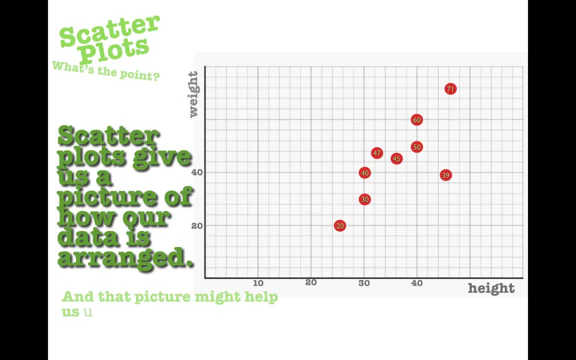 of how the data is arranged. So look at this. We can understand the data. We can understand the data better by seeing that it kind of goes in an upward trend, And what that means in this situation is generally, as children grow up, the taller they are, the more they weigh. 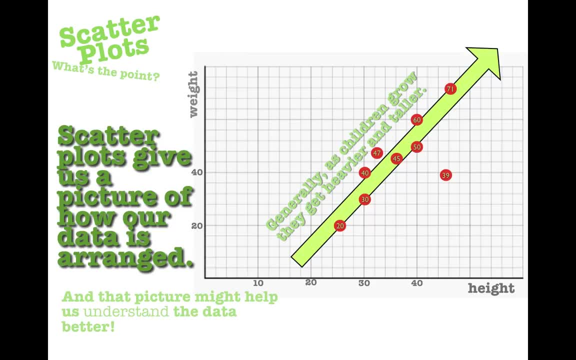 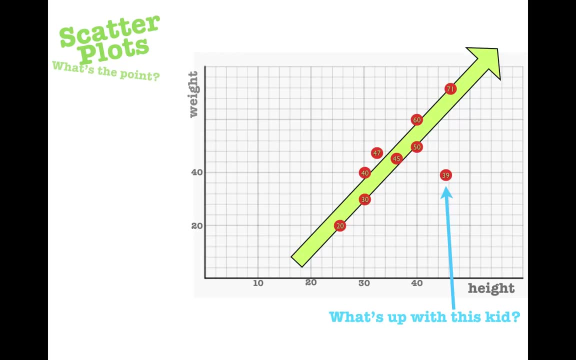 and the shorter they are, the less they weigh, And the scatter plot shows this by the pattern of the dots on the graph. But what's up with this kid? Well, this kid is just special because they're tall, They're the second tallest kid- but they're skinny. 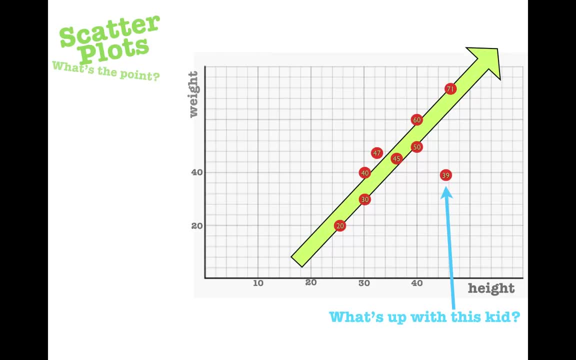 They're the third tallest or the third skinniest or third least weighty child that was measured. This child is what we would call an outlier. An outlier isn't bad, It's just somebody that doesn't follow the general trend of the rest of the data. 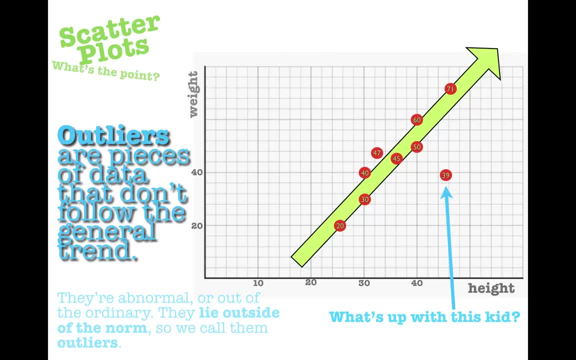 Since this is abnormal compared to the rest of the data, it lies outside of the norm, and we call it an outlier because it lies outside of the norm. This kid's just special, That's all, and it's good to be different, so be nice. 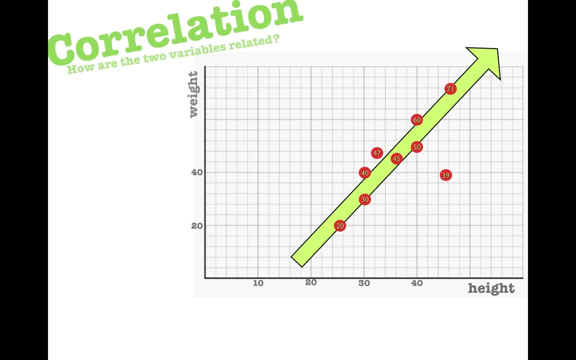 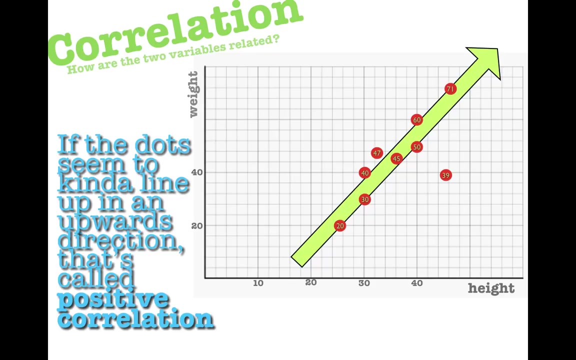 All right. now, when you have your scatter plot, so that the dots make a pattern, either going upwards or downwards, or horizontally or vertically, we call this correlation. Another word for correlation is association, and what we're saying is the two variables in question in this case. 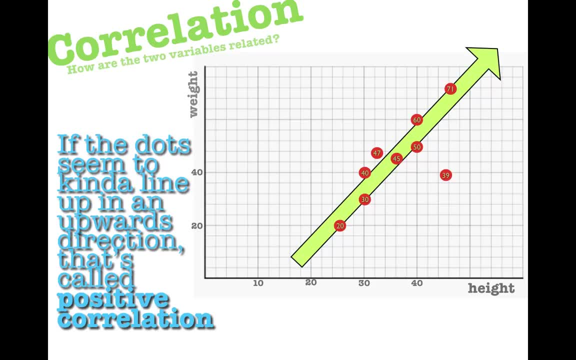 height and weight are related to each other, They're co-related or they're associated. so if the dots seem to kind of line up in an upward direction, that's called positive correlation, like positive slope on a graph. Positive correlation means that as one variable increases,